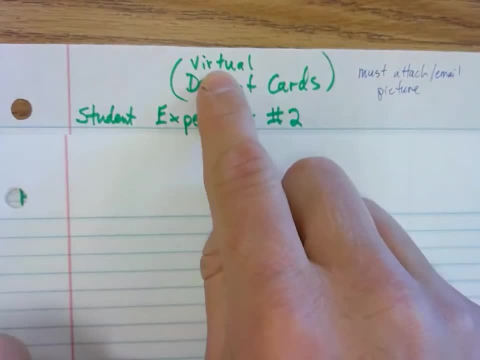 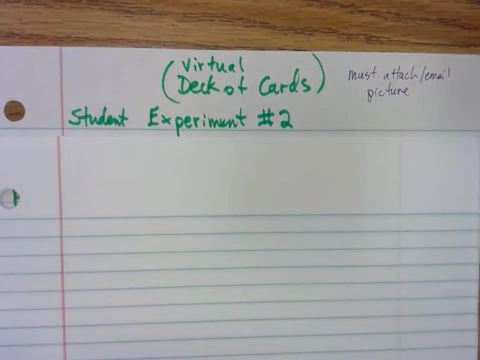 whatnot? cause you don't have a deck of cards. you can type in and search virtual deck of cards and the first little thing that pops up up there on the screen on mine says deck of cards, and just click on that, or you can go to random. I think the one you might want to do is randomorg playing card. 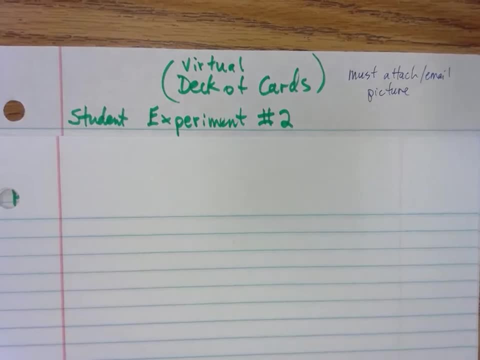 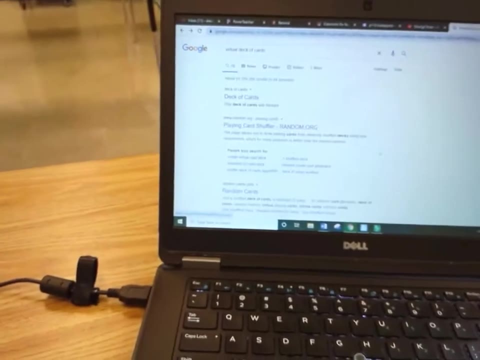 shuffler, Let me just pull it up here and I'll shoot a shot of it on the screen. hopefully Let's see. So let me, let me take it in there and hopefully you can see that. Let's see, can you? 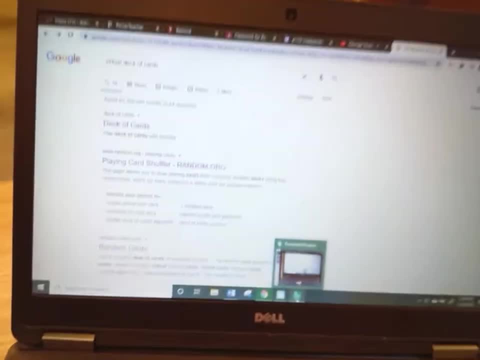 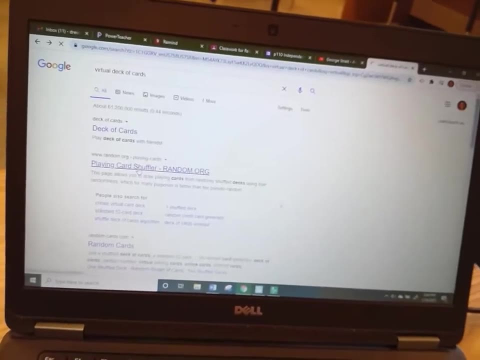 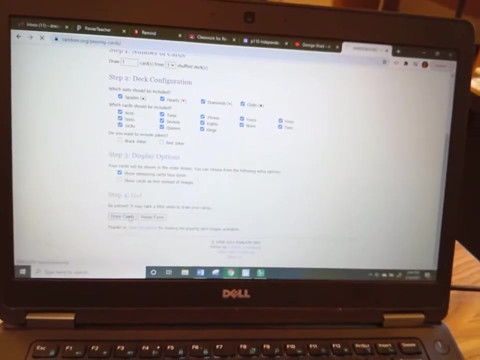 see that. Oh yeah, So right there. second one down says randomorg playing card shuffler. I'm gonna click on that for you and then right here you can just go down. You're gonna do one card from the deck and just go down here and click draw cards and it'll show you So that one's a nine of diamonds. 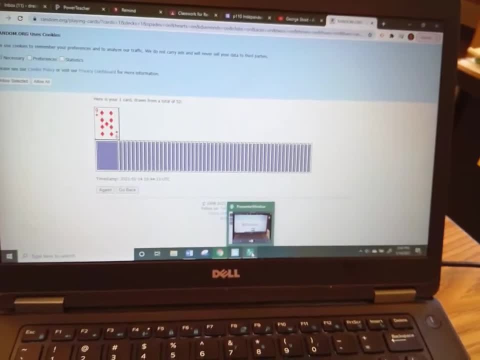 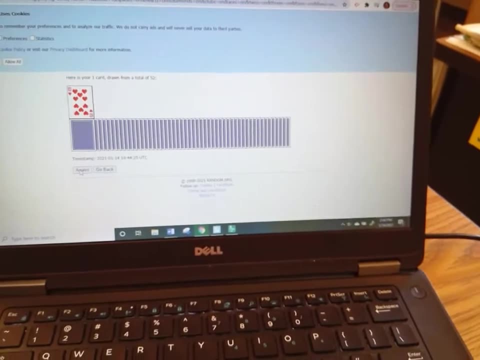 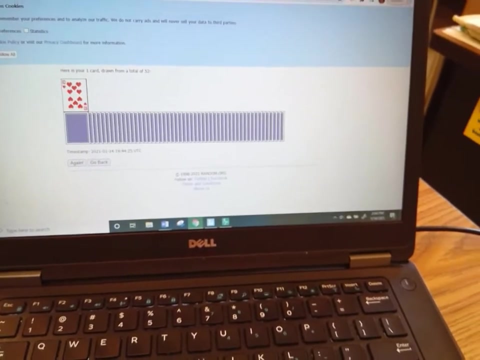 Is that showing up? good? Oh yeah, Then just go again and then six of clubs and hit again and they just randomly pulls the deck card out of the deck. All right, So that's the one you want to do, Randomorg, once you get on there. All right, Let me go back a little, All right? So today, if you, 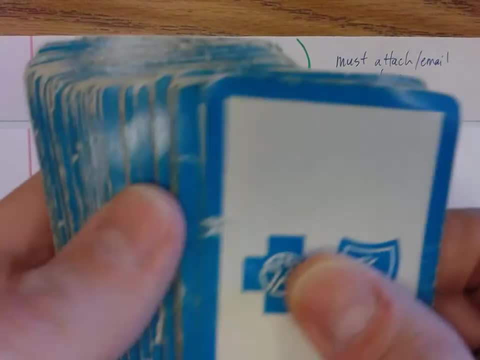 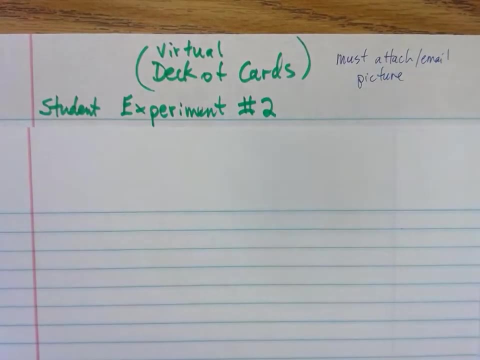 don't have. if you do have the cards, you know, I'd rather- you know it's more fun to do it that way- Actually pull them out of there. This is student experiment number two, and I want to remind you that you're going to have to attach or email me a picture of your work. All right, So now here. 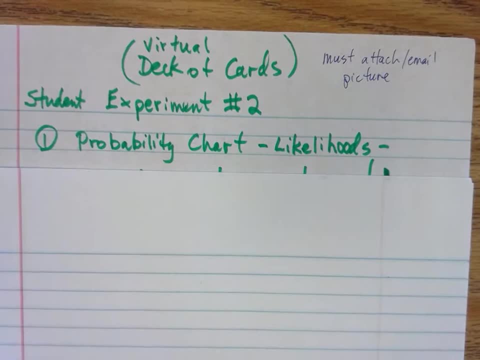 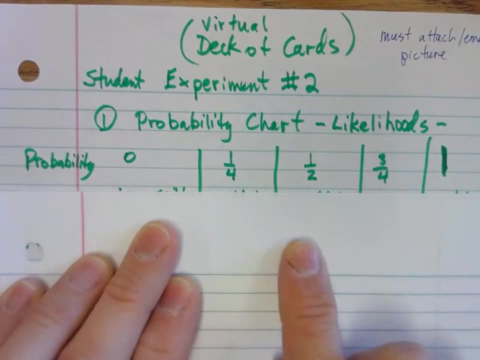 I do want to review this because today we're going to start tying in some of the stuff I did at the beginning about likelihoods with you. So I just want to remind you that on the probability likelihood chart, okay, over here on the left you got a probability of zero, Over here on the right you. 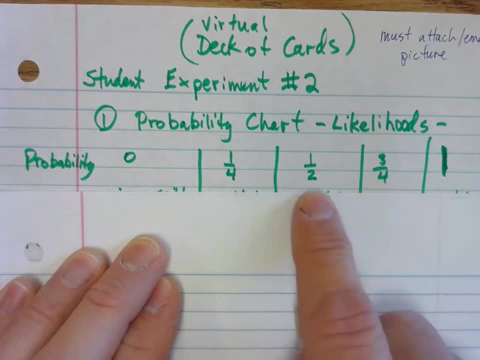 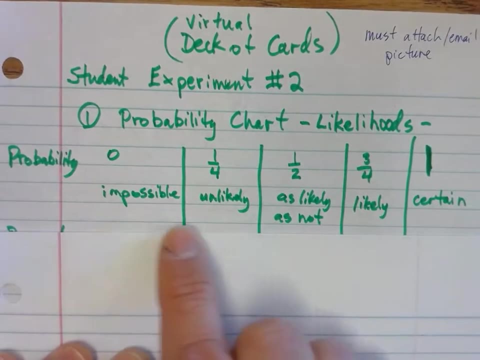 got one. and then you know, these are the ones, major ones in between. You got a half, You got a fourth, You got three-fourths. So the words that go with them are zero, of course is impossible, One-fourth. 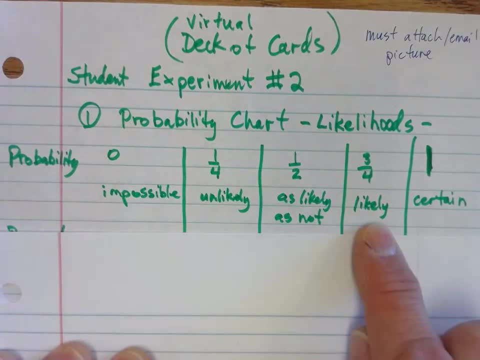 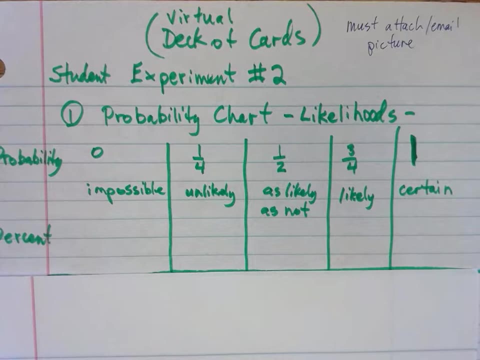 half would be as likely as not, Three-fourths is likely and one, of course, is a hundred percent as certain. So let's come down here and I'm going to add these percentages in. You're going to have one of these papers, if you can print it off. If not, you just have to write it down, but if you 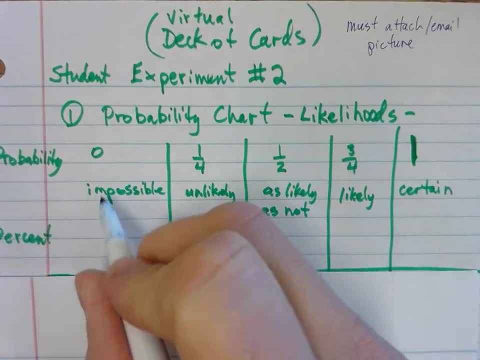 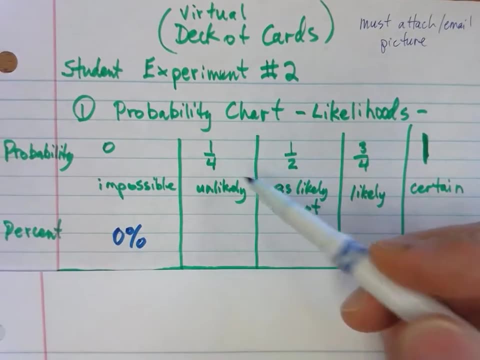 can print it off. of course you can do the same thing. So impossible of course. percentage-wise the probability is zero, but the percent would be zero percent. Unlikely's probability is one-fourth and the percent for unlikely of course would be twenty-five percent. Half, of course, is the 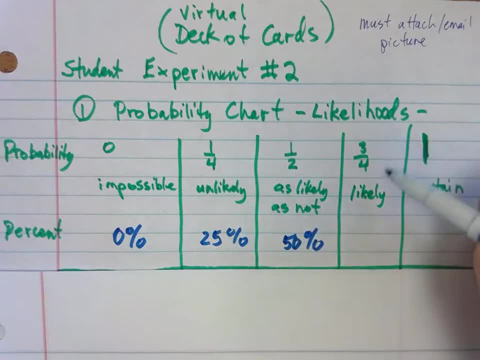 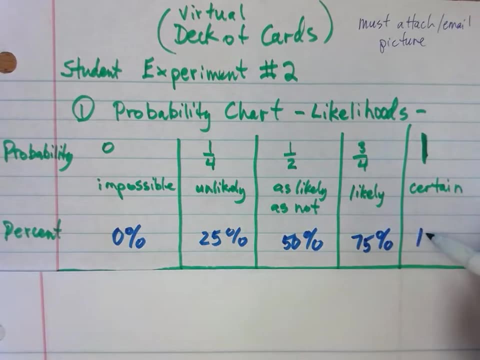 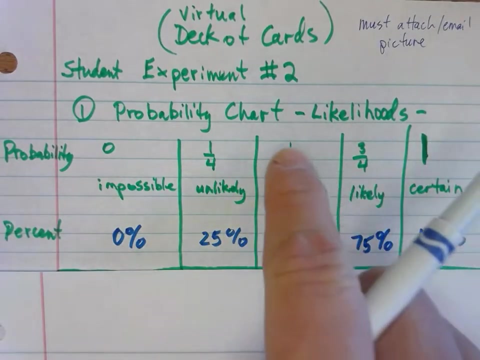 probability, The percentage would be fifty percent, Three-fourths for likely as a percentage would be seventy-five percent and of course certain is one. That's the probability, So that would be a hundred percent in percentage category. Now, remember these things: the fractions are the. 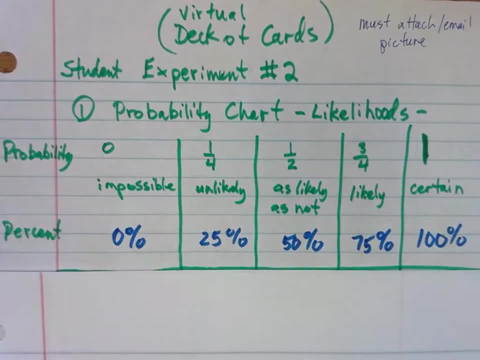 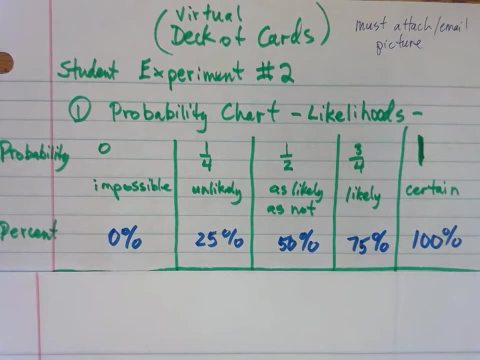 probability, Then you can take that probability and turn it into a percent. So you might want to get all that down. Impossible, unlikely, as likely as not likely, certain. If you need to hit the pause button right there, you can pause it and do whatever you need to do. okay. 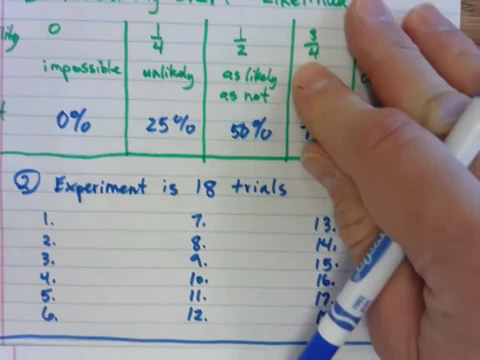 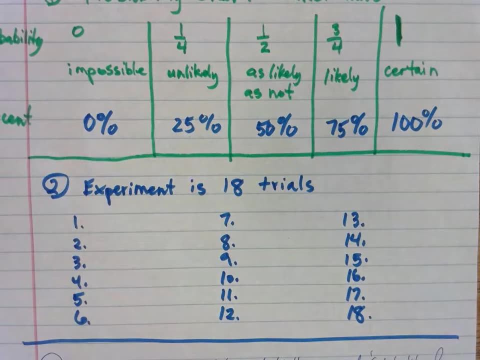 I'm going to move forward. So the next thing we're going to do here is: you're going to do an experiment, and I'm going to do mine right here with you too. We're going to do an experiment. The other day, I did one that had 24 trials and I just wrote them down and everybody freaked out on me. 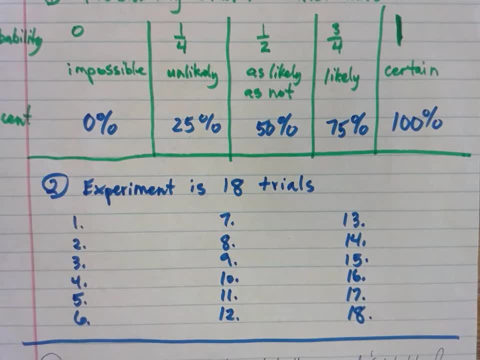 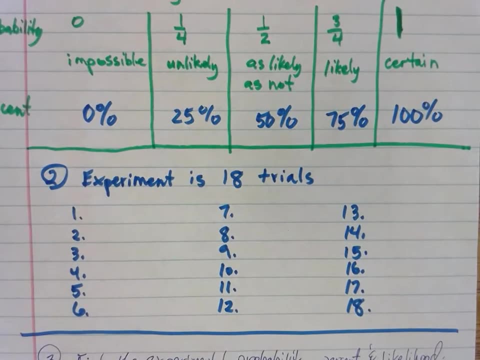 okay, So today we're going to do an experiment with 18 trials, and I'm actually going to write the cards down so you can have a real good knowledge of how this works, and then you won't be freaking out, Hopefully, like some of y'all were the other day. So I've got my deck of cards here. 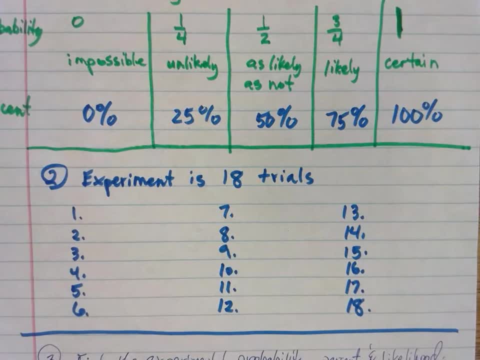 and I'm just going to pull it out, and I'm just going to pull it out, and I'm just going to pull them out one at a time and I'll show them to you and then we'll write them down, okay, So my first. 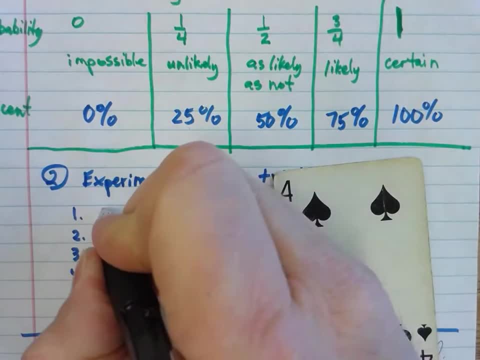 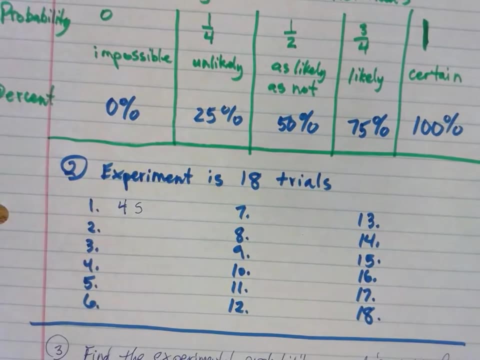 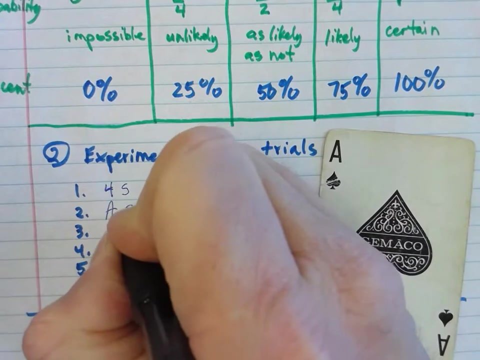 trial, I got a four of spades. So I'm going to write down four S, that stands for four of spades. all right, I'm going to stick that joker back in there and shuffle them around a little bit and let's see what else I got here On my next one. hey, I got the ace of spades. okay, Ace of spades. 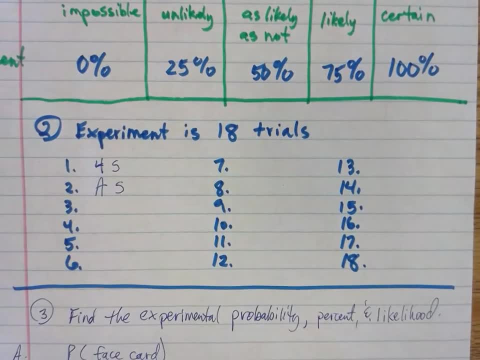 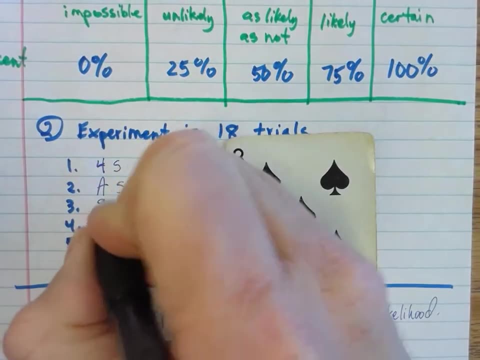 all right, I'm going to stick that one back in there, shuffle them around a little bit, shuffle, shuffle, shuffle. And my next one: oh my gosh, another spade, eight of spades, all right, And shuffle, shuffle. 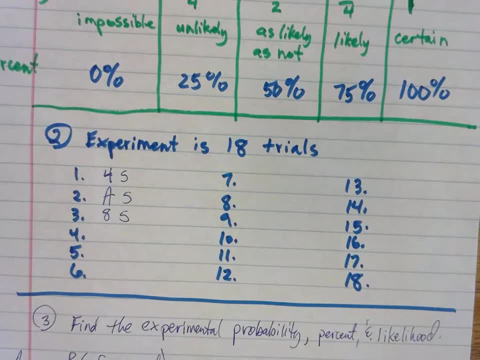 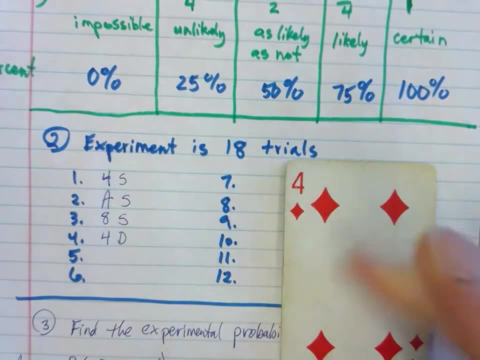 shuffle. My next one is: let's see, come on out of there, What we got: A four of diamonds. So I'm going to write down four D, four of diamonds. all right, That one goes back in the deck. 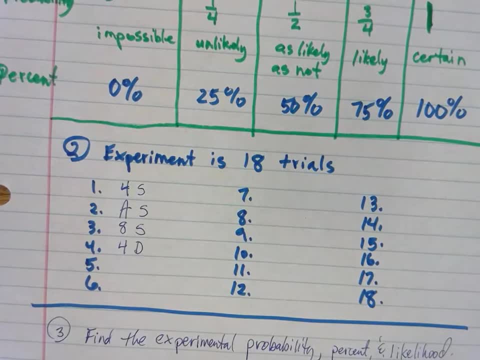 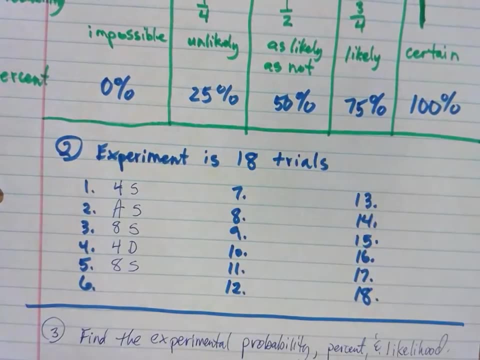 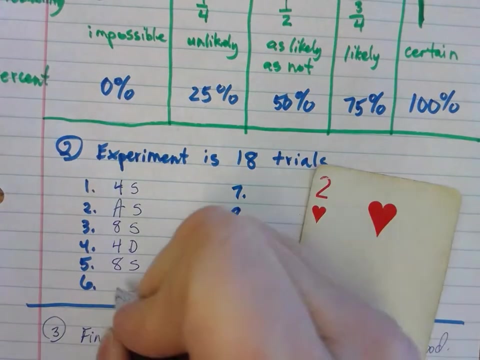 shuffle them around a little bit. And my next one: oh gosh, another eight of spades. how in the world am I getting all these spades? All right, shuffle them around a little bit. let's see what that one is. Two of hearts, two of hearts. So I'm going to write down two H for that. 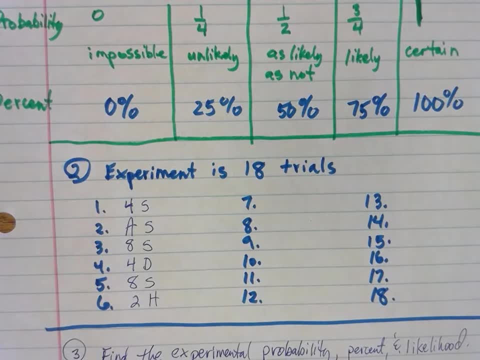 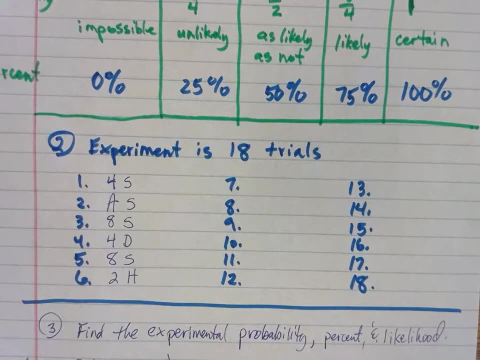 two of hearts. All right, I'm going to shuffle them real good this time. So I've done six trials and if you need to make sure you get all those written down while I'm shuffle them around, you go ahead. So far, okay, I've got a lot of spades. I've got eight. a couple of times. 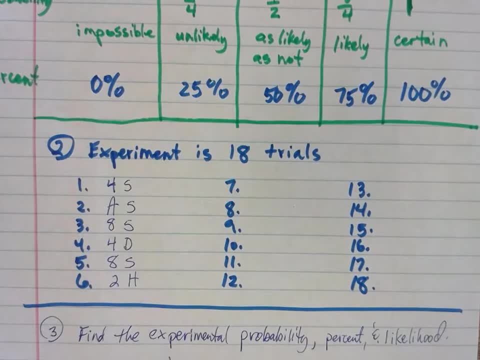 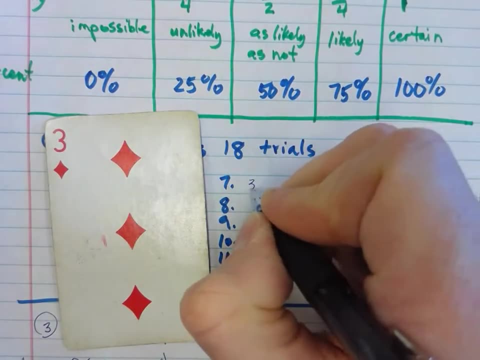 four a couple of times hadn't got a face card yet. I got three, three, four. all right, That's times I haven't got a face card yet. I can't believe that. all right, let's see what we're gonna do here now on the next ones. so I got a three of diamonds. 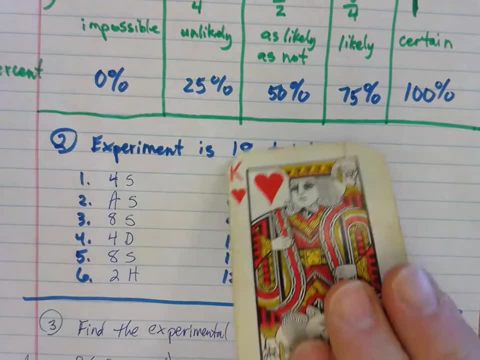 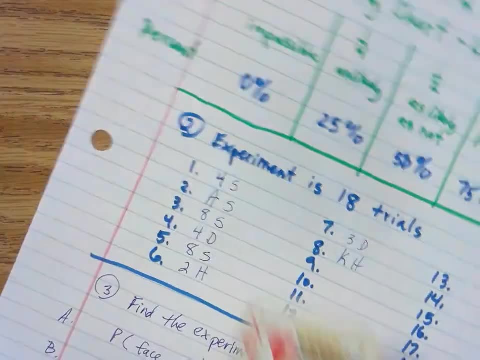 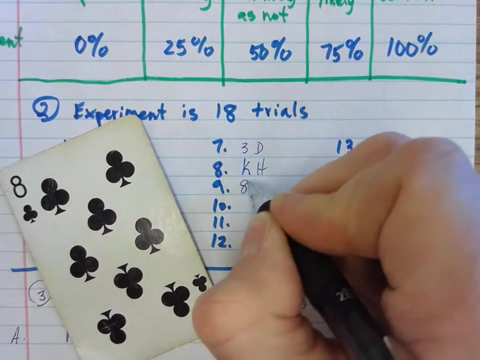 check it back in there. I got: ah, there's my first face card. okay, I got the king of hearts. put K hearts. let's see what we got right here. eight of clubs, all right, I'm gonna smudge them around a little bit. let's see what else we got. 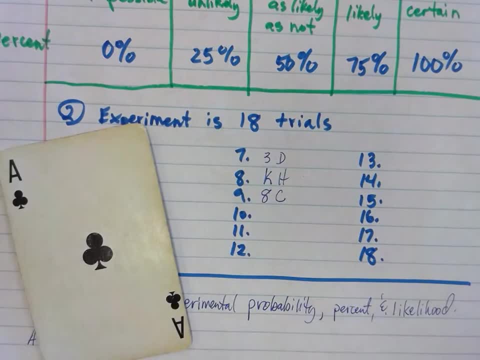 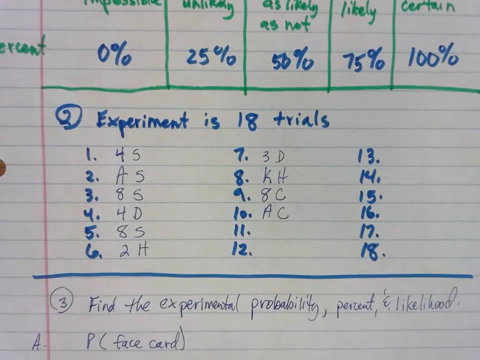 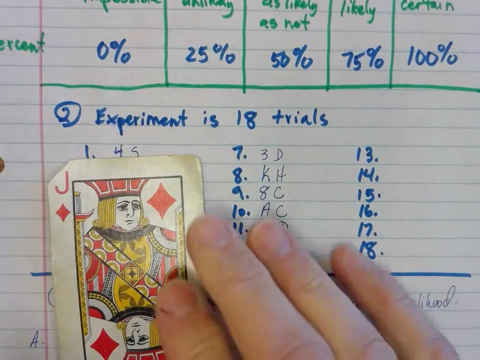 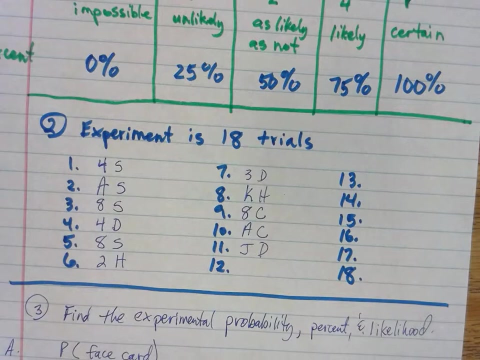 here about that one ace of clubs. let's see, you got a another one down here. hey, there's another face card, jack of diamonds, and let's see what number 12 is gonna be here when I pull this one out. hey, jack of clubs. hey, wow, I got some face card that go around, all right. so from my 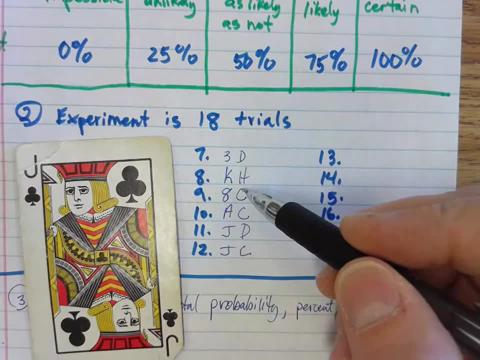 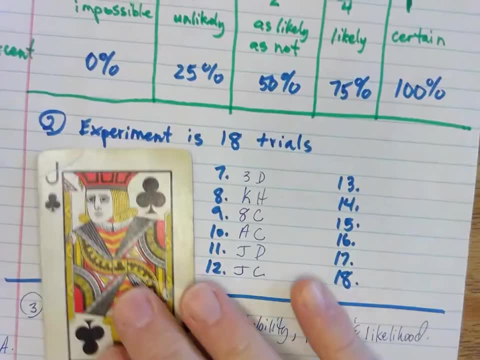 number seven: I got a three of diamonds, king of hearts, eight of clubs, ace of clubs, jack of diamonds and jack of clubs. so right there, I got three face cards out of that little run, all right. so so far I've done 12 trials and now I've got. 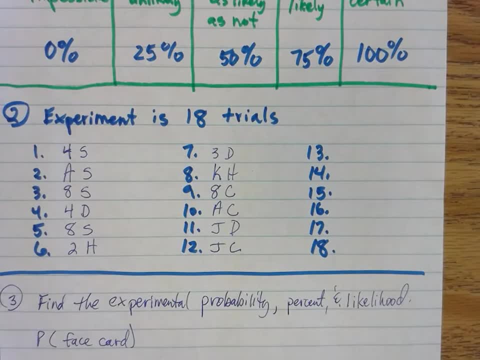 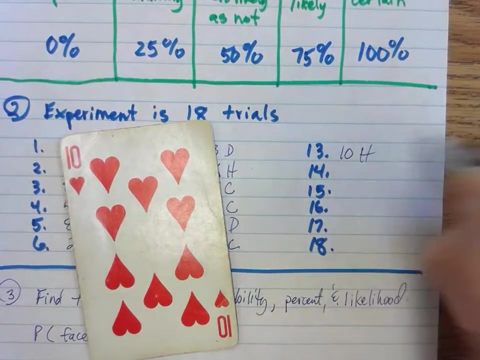 six left so you can go ahead and make sure you got all that written down. well, I'll take a little shuffle here and we're going to head off to our last six trials and experiment. all right, I got them all shuffled up and here we go, ready to go, and I'm pulling out that one. that's ten of hearts. take it back in. 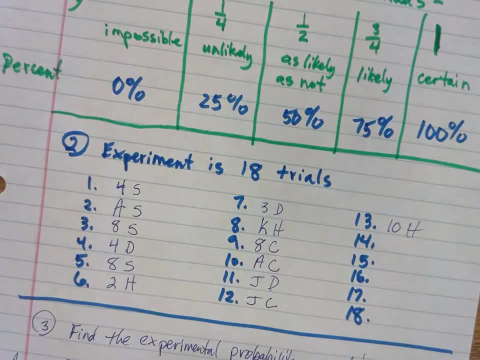 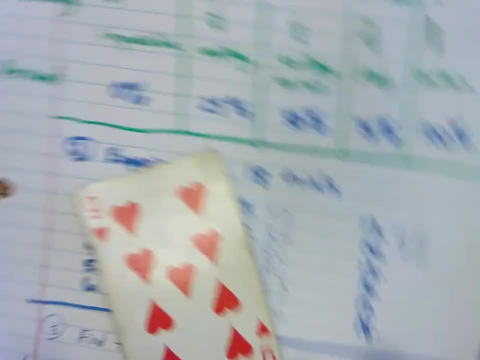 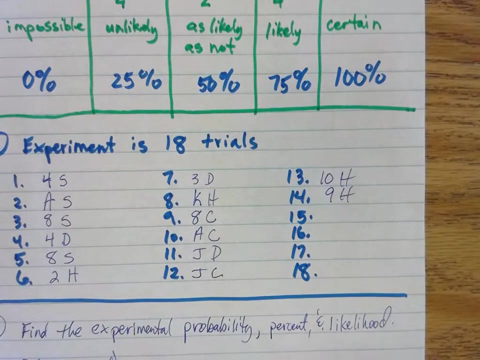 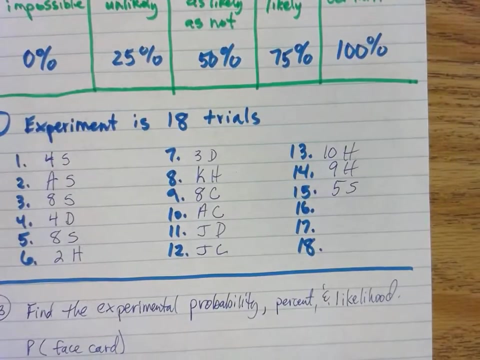 there. let's see, we're gonna get nine of hearts. oh gosh, ten of hearts, nine of hearts, and we're connections gonna be the eight of hearts. so ten of hearts, nine of hearts. let's see what we got down here at this in five of spades, all right. 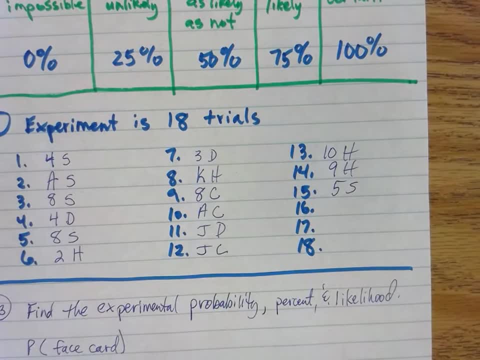 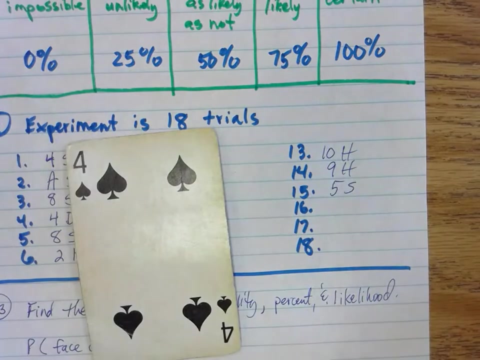 I'm gonna shuffle them around one more time. got three trials left. okay, this is an experiment. this is not theoretical. okay, we are actually testing this out, getting some experimental results here. three more: all right, I got them all out here and ready and I'm gonna pull this one right here. four of spades: man, we have gotten a. 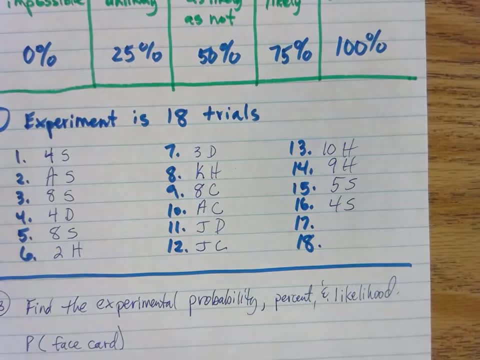 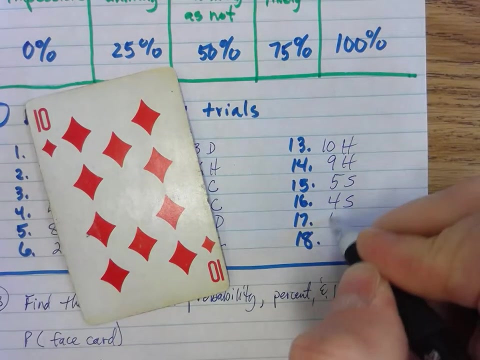 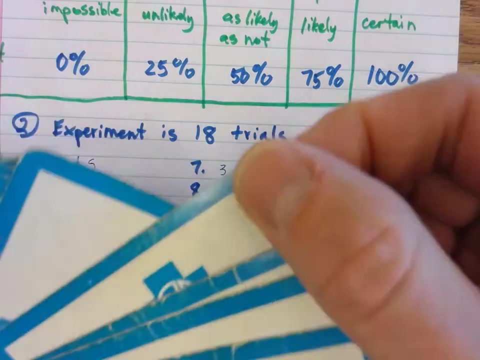 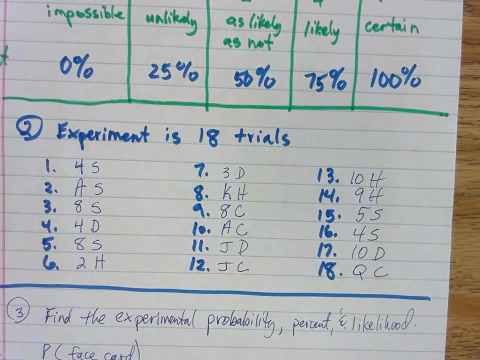 bunch of spades, that is for sure. got lost one there. let's see what we're gonna have left. okay, ten experiment is going to be this card. right here got me another face card, queen of clubs, all right, so now my pulling is over again if you don't have a deck of cards. 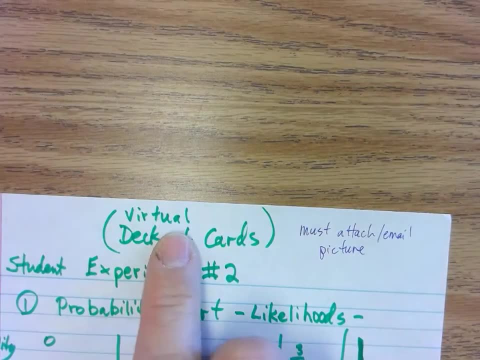 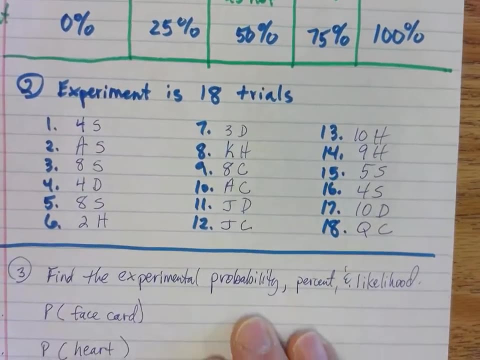 you need to go and type in virtual deck of cards on your search bar and then choose that one that said random. all right, but there's mine. I have my deck of cards. so there's my 18 trials. now, down here at the bottom, I'm gonna do another three trials. 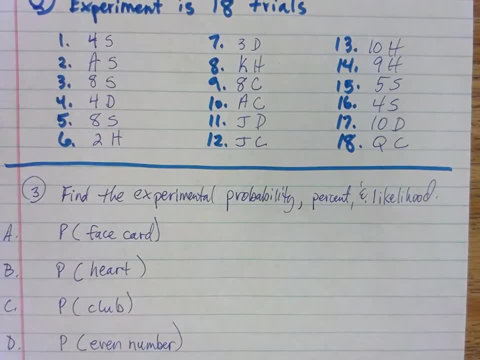 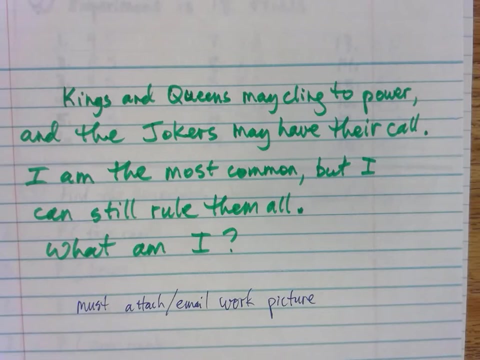 the bottom. I've got some questions for you to answer about these trials and I am gonna ask a little riddle question before we get into that. so let me bring my friend back. in. hello people. all right, today's riddle is about kings and queens. alright, since I was born in jolly old England, I know a little bit about kings. 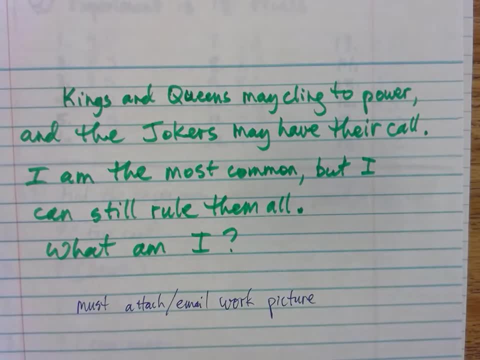 and queens. so let's see what you've got up here on. it say: kings and queens may cling to power and the Joker's may have their call. I am the most common, but I can still rule them all. what am I? hmm, there's a good question. 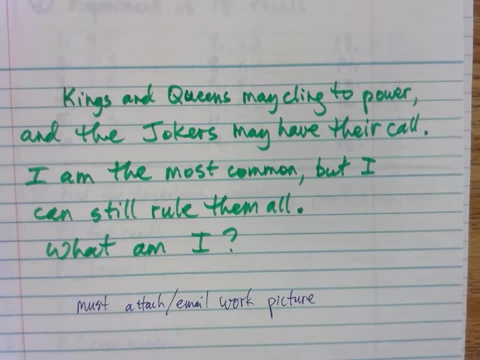 kings and queens may cling to power and the Joker's may have their call. I am the most common, but I can still rule them all. what am I? oh, I think I know. if you think you know, don't forget to email in your answer, or you can write it, you know, and send it in, or whatever in today's work. he said: 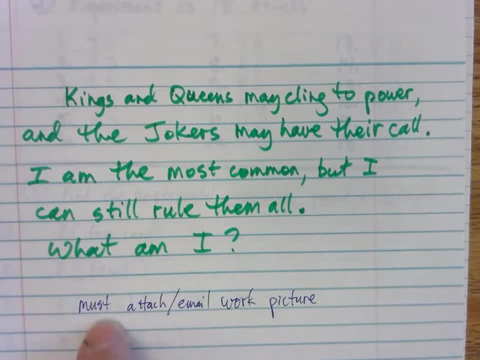 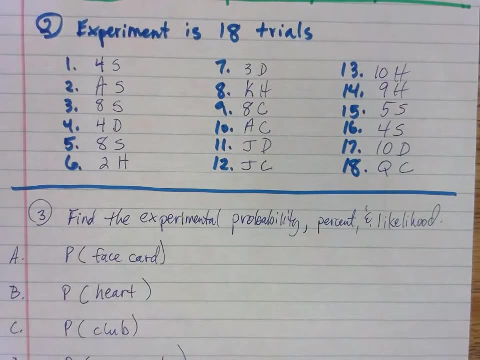 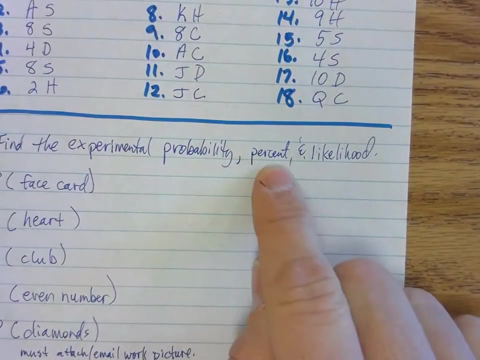 make sure you attach an email at work picture all rights. and don't forget to do that. you must attach an email, your work picture. until next time, friends. ciao for now. okay, now we're gonna find some probabilities, we're gonna turn them into percentages and then we're also going to 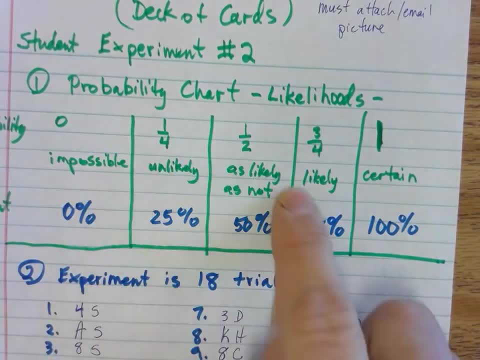 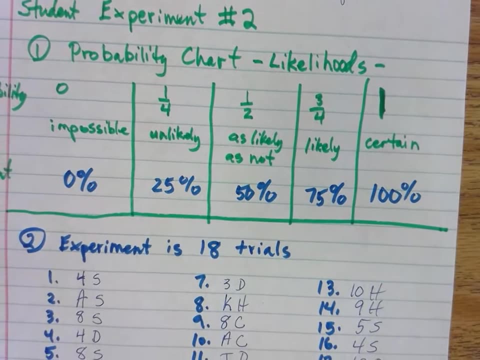 go back up here to the top, to the likelihood chart and decide which one of of these words would be the one that would be most close to it. okay, would it be impossible? unlikely, as likely as not likely or certain. so I'm gonna do a couple of these with you and hopefully that'll have you going in the right. 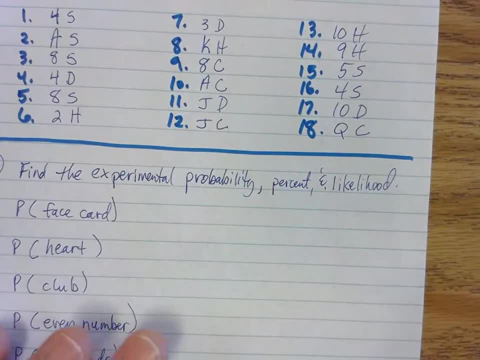 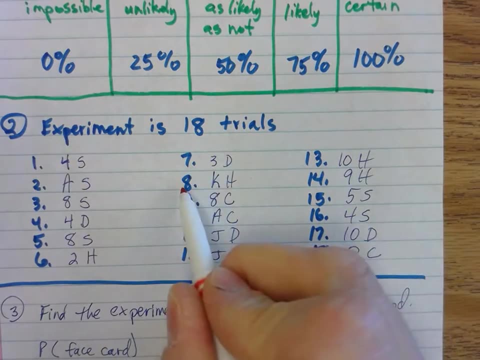 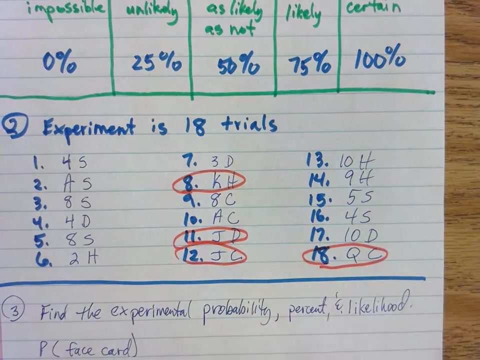 direction. okay, so let's do our face card. so if I go back up here and I look at the face cards I drew out in my trials, okay, I got a king of hearts, a jack of diamonds, a jack of clubs and a queen of clubs. so I got one, two, three, four. now 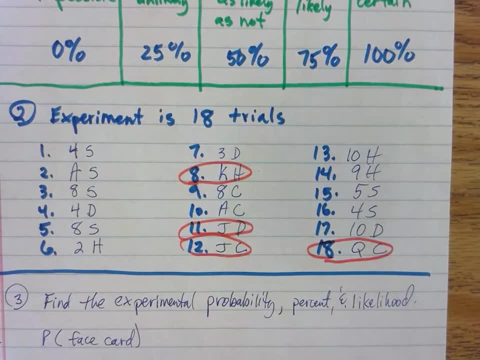 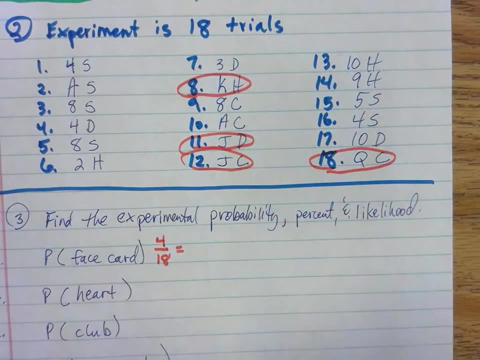 that's four out of how many, and you better not tell me fifty two, four out of how many. that's four out of eighteen, because we did eighteen trials. I can simplify that and divide them both by two and take it down to two, ninths and I 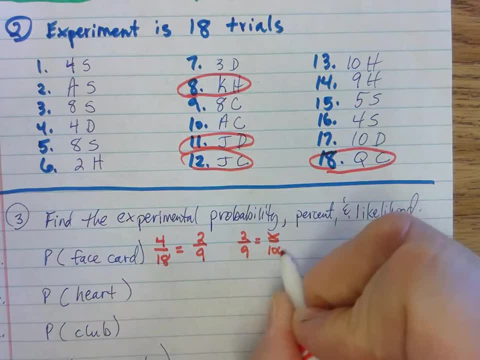 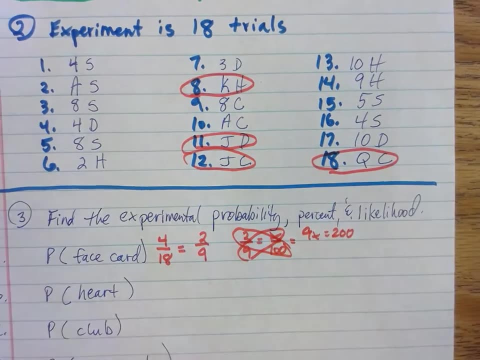 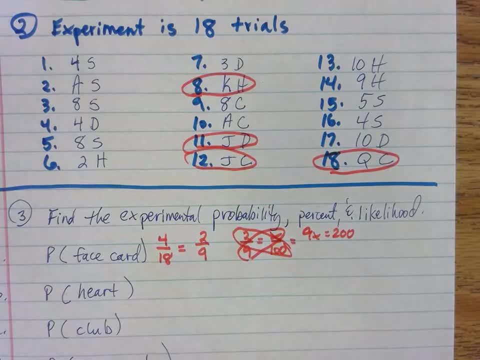 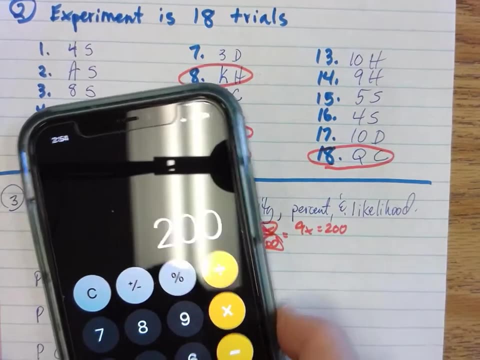 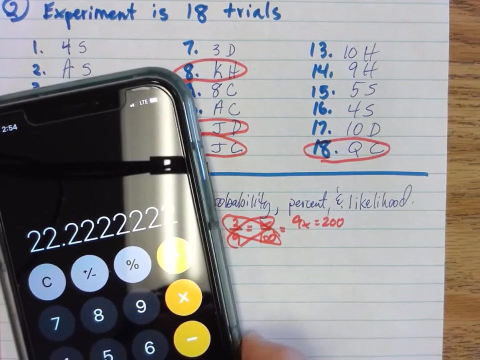 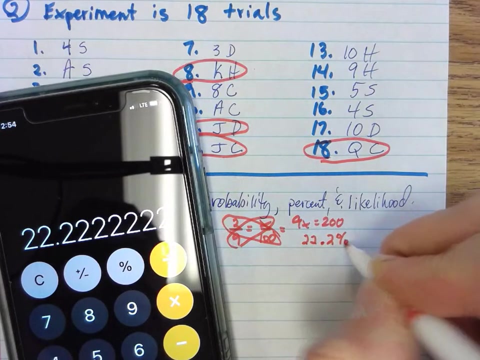 divided by 9. let's see what we come up with on that 200. let's got a lot of reflection on 200 divided by none. it looks like I'd be 22.2%. okay, I've got that that. Again, make sure you go to the nearest tenths place. So I've got the. 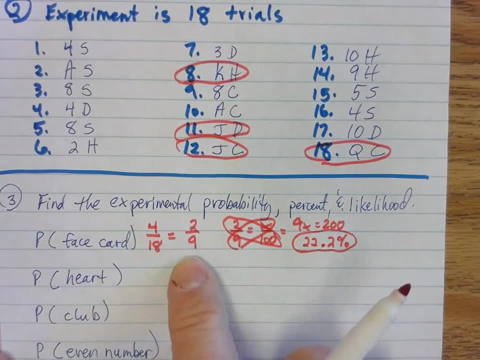 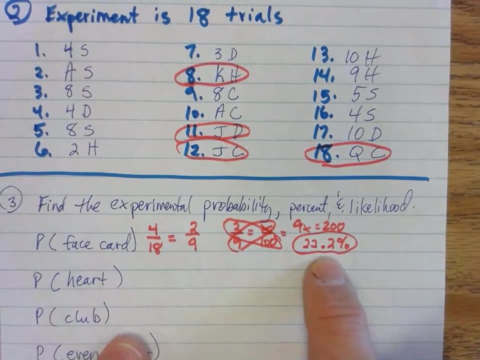 probability was two ninths. So there's that, answer number one. I got the probability always a fraction. Answer two is the percentage. Now, if I take that up here and look at the likelihoods, which one of these likelihoods is closest to? 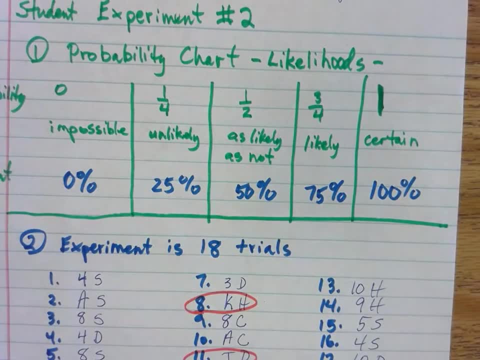 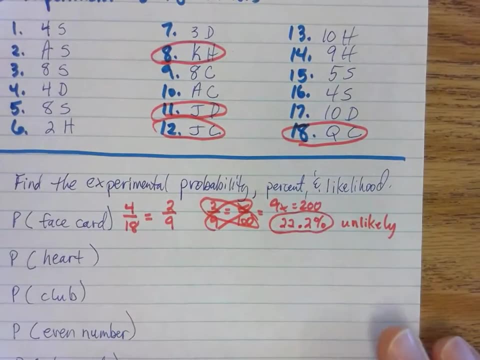 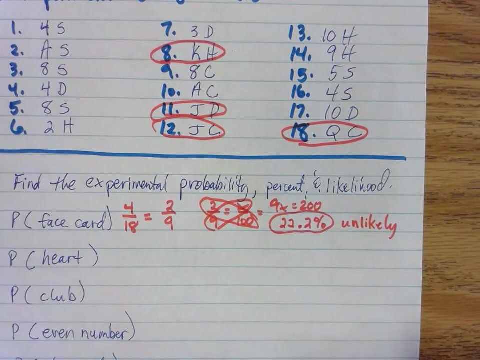 22%. I would say unlikely. Okay, so that would be the word I would put. with that, I got a feeling you're gonna have a lot of them that are down there on that end. Unlikely. Let's see about hearts, though. I don't remember how many hearts I got. I. 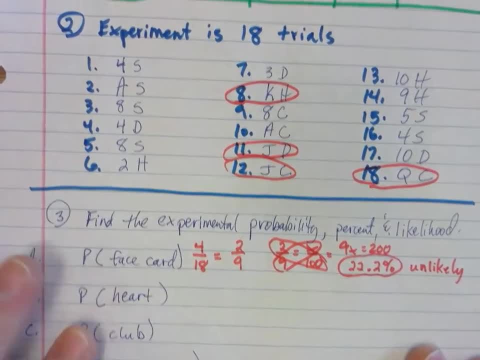 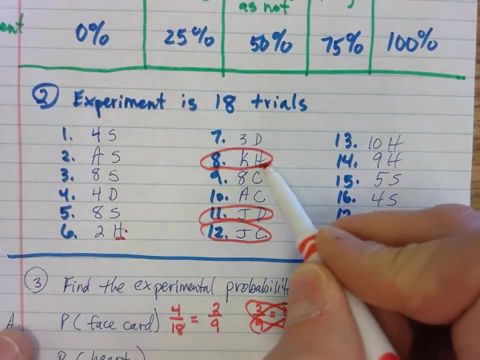 felt like I was getting a lot of spades at one point. but let's see, So let's find out the probability of hearts. So I got a heart there. Let's see, can you see that? So I got a heart there. There's one heart, two hearts, three hearts, four hearts. So 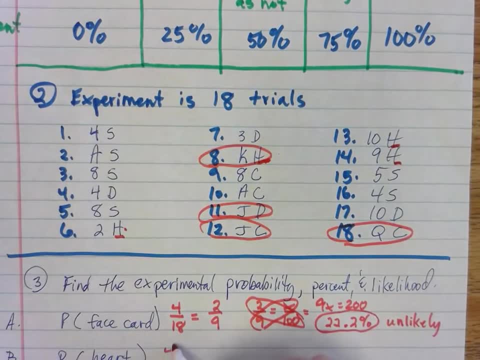 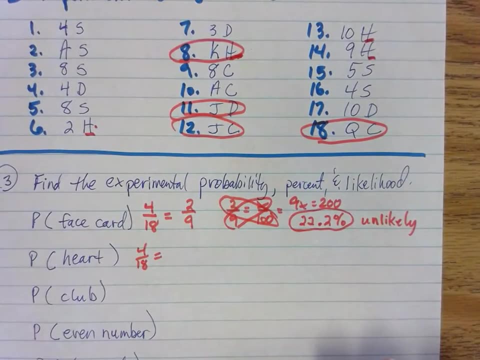 again. hey, for me that's gonna be the same answer. Okay, all the same stuff, because I got four out of eighteen, Okay, Four hearts out of my eighteen trials, Not four out of fifty-two. Four out of eighteen, All right. again, that would be two nights, which would be 22.2%, and the 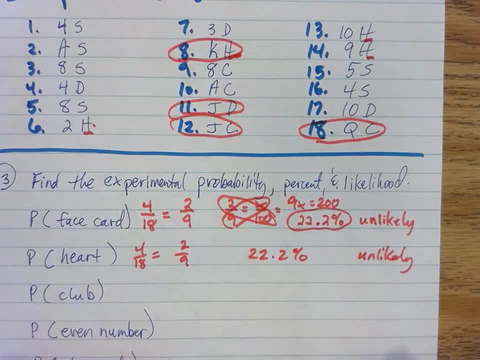 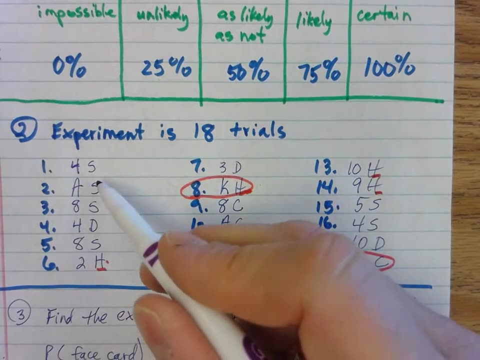 word again. still, of course would be unlikely. All right, let's do clubs real quick. Let's see how many clubs I got. I'll do that in a different color here. So clubs, I didn't get any clubs there. I got one club, two clubs, three clubs. 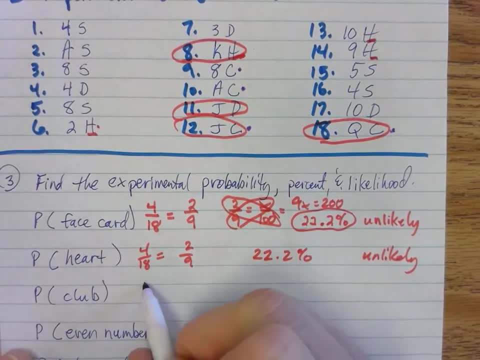 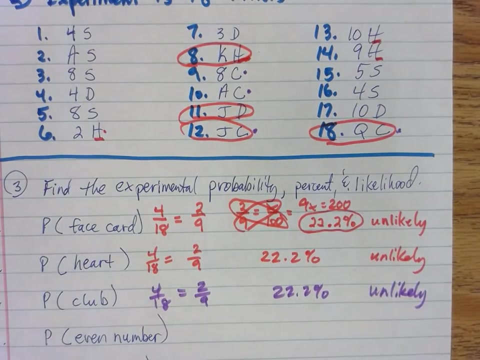 four. Oh, my lord, getting the same answer again. So alright, so all that stuff is gonna be the same. How about them apples? You may have this same habit than you. I don't know everybody It's gonna be different. maybe yours are gonna be like mine. All right, let's do even numbers, okay, Even numbers. 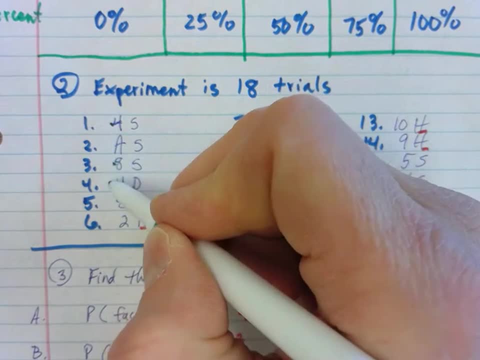 So we got one, two, three, four, five, six, seven, eight. Omph, There goes our new club: Five, six, seven, eight, So five That's mine. So now we got three, So that's a five. 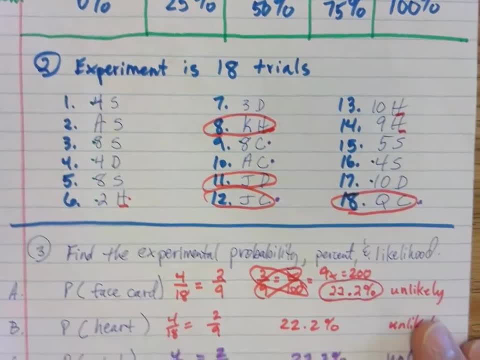 So what's the number of the poальное we caught? So we got our number. four, five, six, seven, eight, Alright, a level here. we got Ugh Four, all right, so I got eight even numbers. this one's gonna be a little bit. 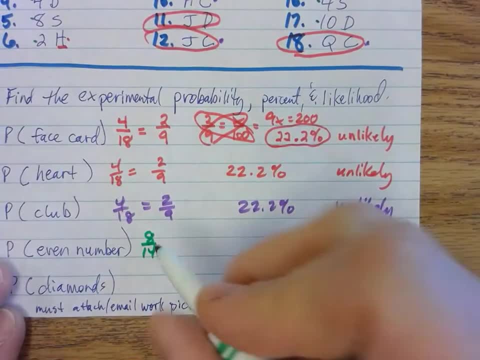 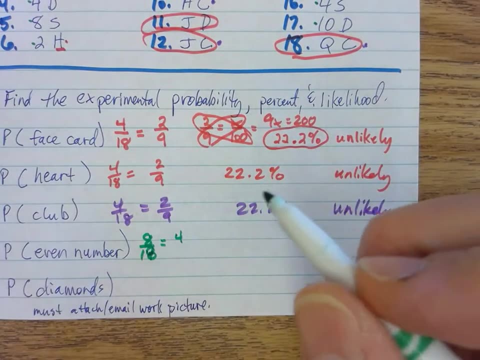 different. eight even numbers out of 14, so eight, fourteenths, of course. if I divide both those by two, that takes that down to- I'm sorry, not eight fourteenths, eight, eighteenths, sorry. and if you divide them both by four, that takes it. 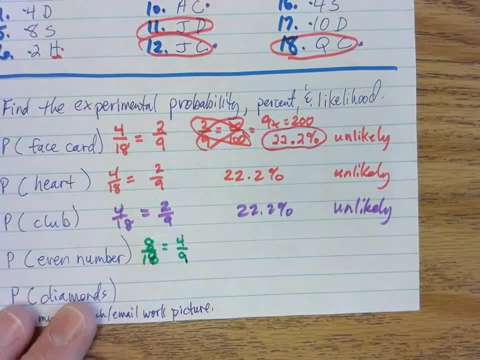 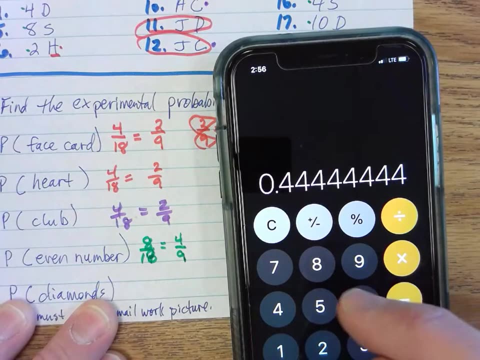 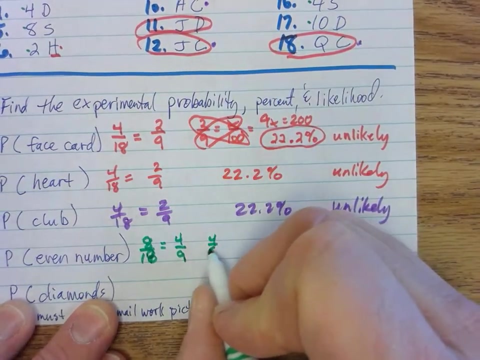 down to four ninths, okay, and if you do four divided by nine, four by nine, that would be in. multiply that by 100, of course, that'd be forty four point four percent, okay. so four ninths equals X over 100, and that is gonna give me forty. 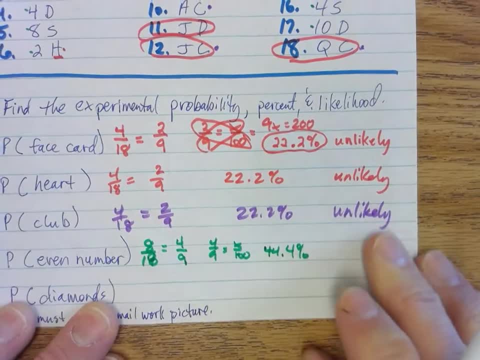 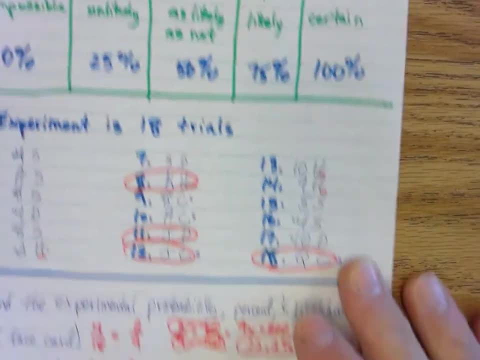 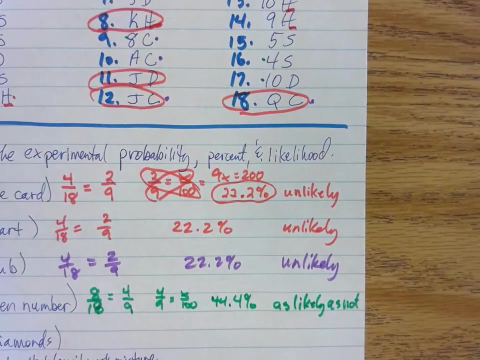 four point four percent, and if you do forty four point four percent, of course that one's a little closer to that than it is to that. so as likely as not would be what we're doing here. all right, that's probably enough. I could do diamonds, but I don't want to keep you. 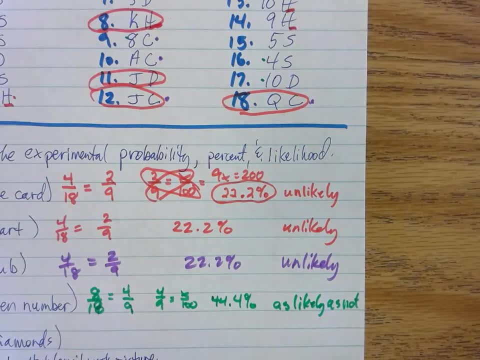 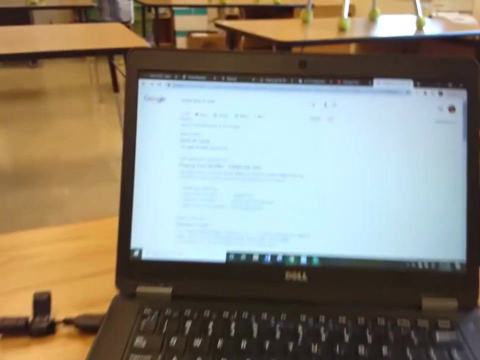 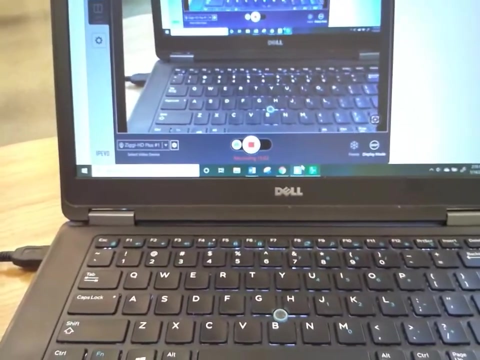 guys on here longer than 15 minutes, so therefore, I believe that's all we got for today. sports fans, and I'll just hit on some of the stuff again real quick. let me go back. all right, let's grab that one any way again, if you don't have a deck of cards. 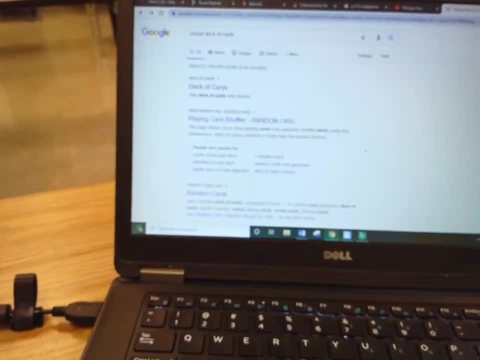 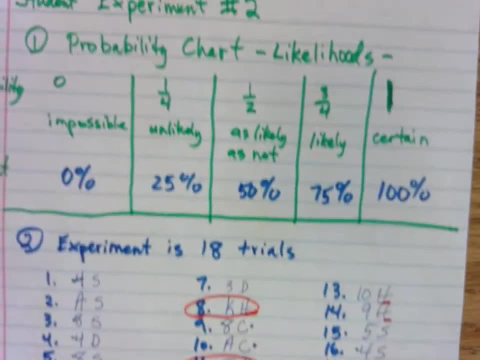 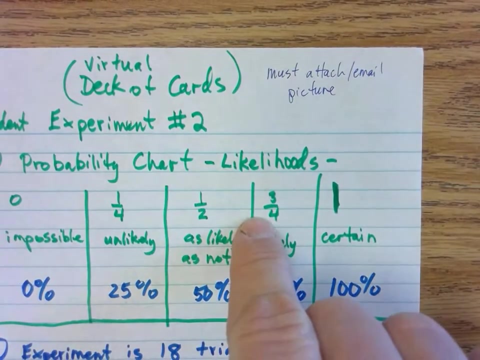 make sure you do that. okay, type in virtual deck of cards and unpick this second one down here that says playing card shopper, random model, and then you take it from there. all right, I must have a picture. Attach your picture, Email your picture. Okay, your results are not going to be like my results, okay, 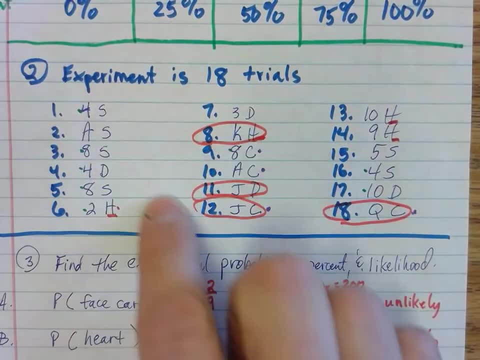 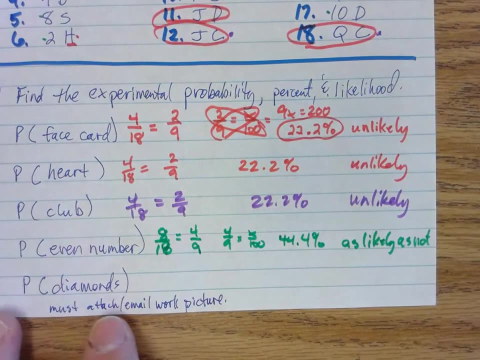 My trials are going to be different than your trials, So make sure you write down all your trials, Answer all your questions down here, Make sure you get the probability, the percent and the likelihood And make sure you attach the picture or email the picture. 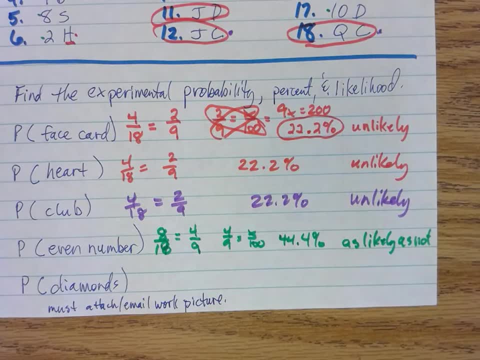 because there's not going to be anything for you to type any answers in today. I'm just going to look at just your work pictures, okay, Okay, so hope you have good success with your cards and don't have no ace up your sleeve. 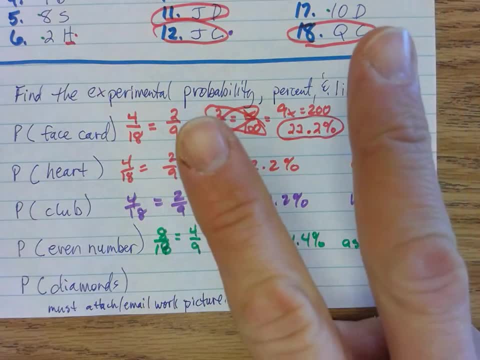 All right until later. Ciao, for now, baby Peace.